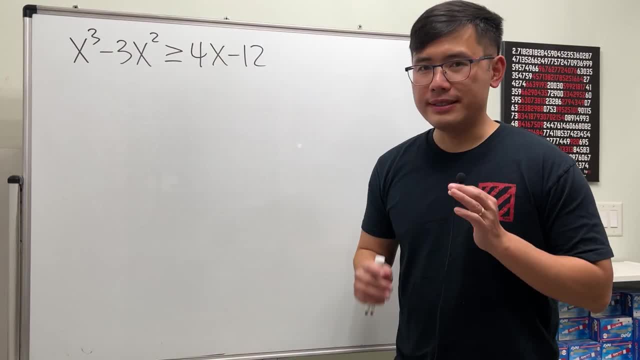 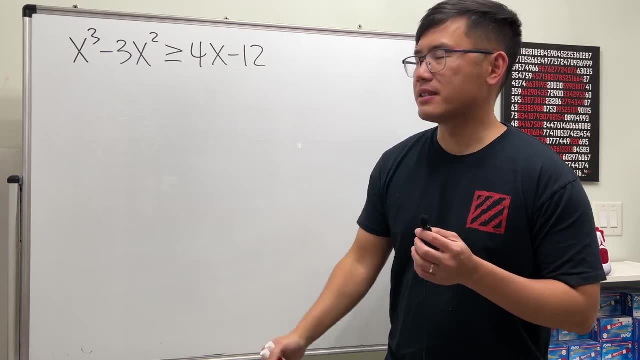 Okay, we will solve this cubic inequality. Well, let's do it the safe way. Let's move these two terms to the other side. Be sure you make one side equal to zero and then factor it and then do the same chart. So here we go. Right, here we have the x to the third power minus 3x squared. 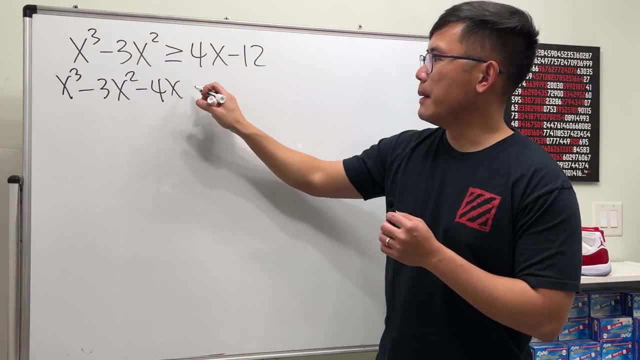 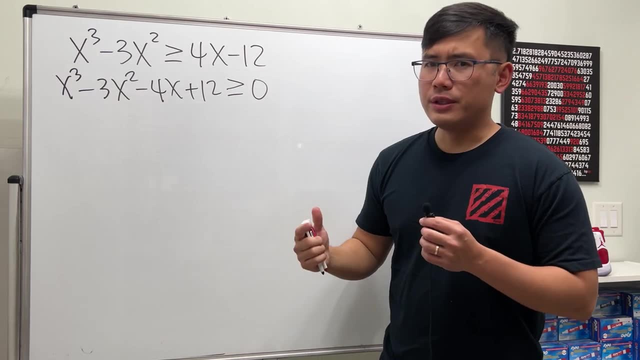 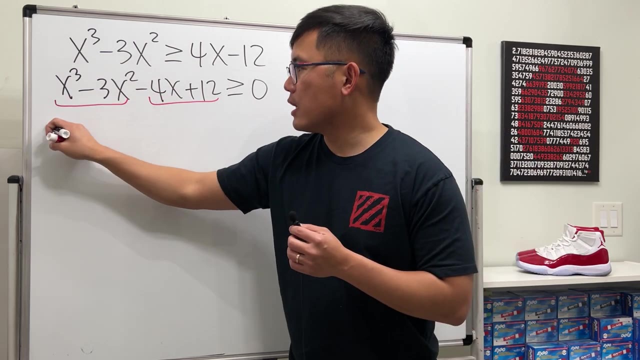 and then this will be minus 4x and then plus 12. And this is still greater than or equal to zero. Now here we have four terms. So it's a good idea to try factoring by grouping first So these two terms and these two terms. Here we can factor out x squared and then we get x minus. 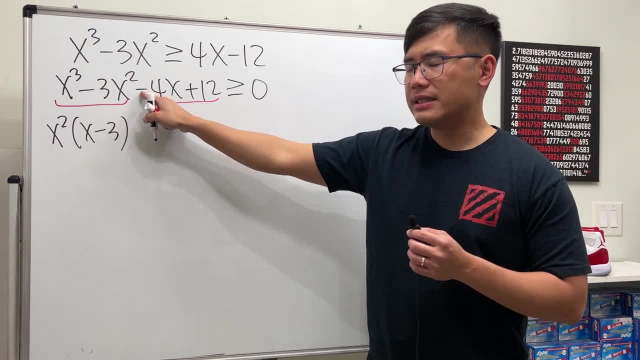 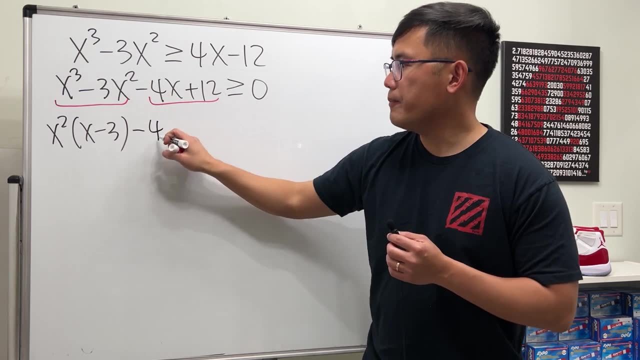 3 here, And then you see, here we have a minus sign in between. So go ahead and write that down right away And look at the 4 and 12. We can factor out 4.. So put that 4 down and that will. 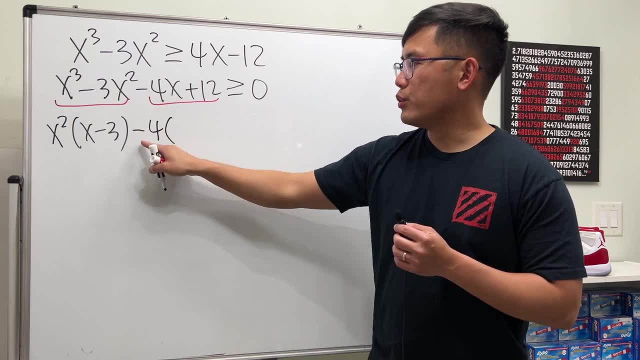 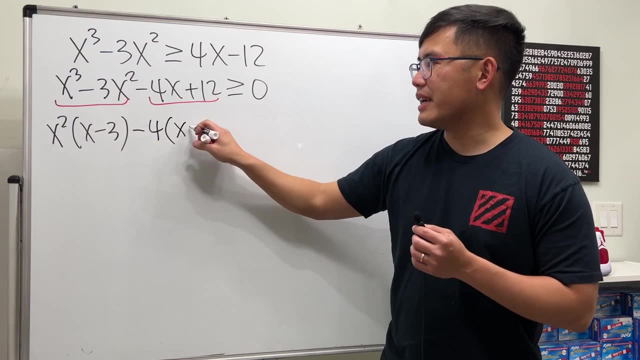 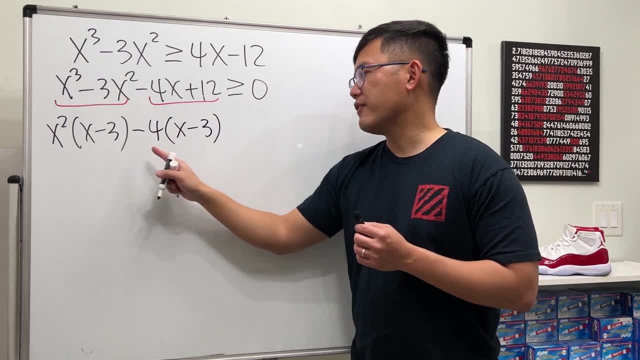 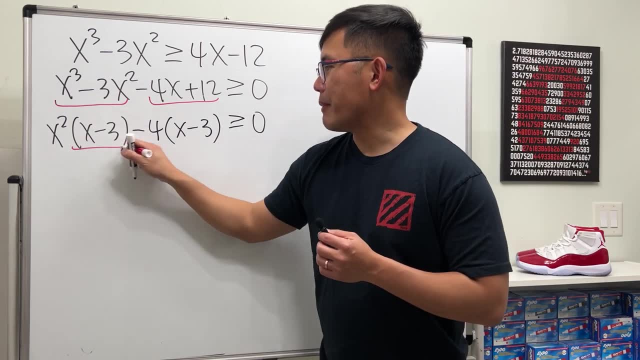 So it's negative 3. Just go ahead and do 12 divided by negative 4. We get negative 3. Same thing, And this is still greater than or equal to zero. Now, this and that they are the same thing. 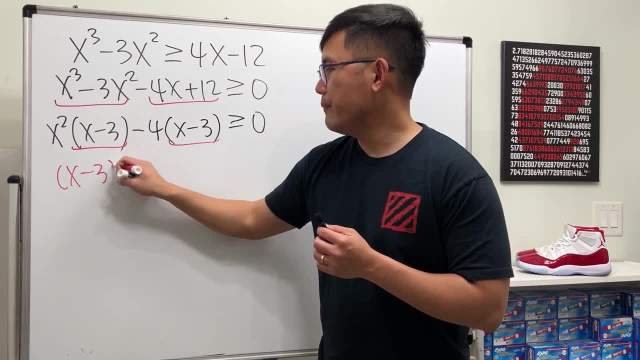 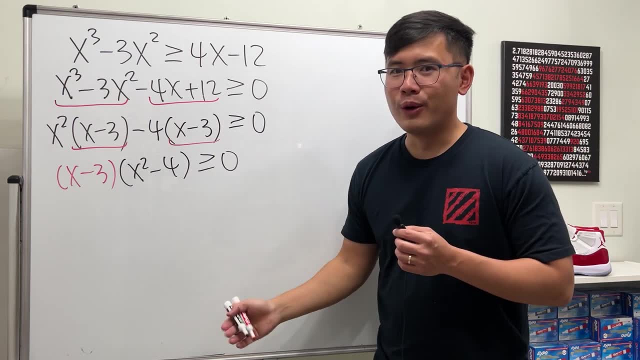 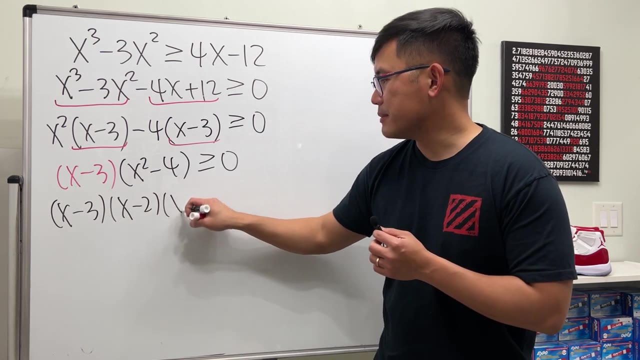 So we can factor that out. So we get x minus 3 times x squared minus 4.. And this is still greater than or equal to zero. Can we factor more? Yes, this thing right. So, as you can see, we have x minus 3 times. this is x minus 2 times x plus 2.. 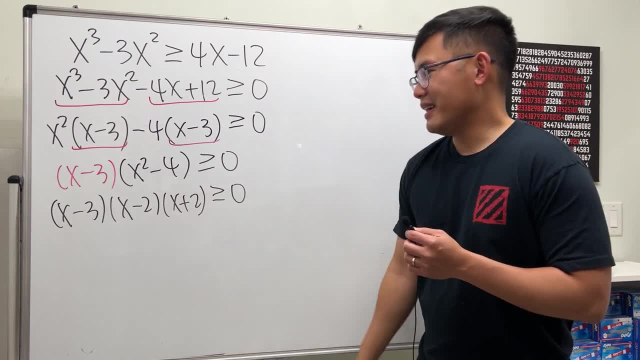 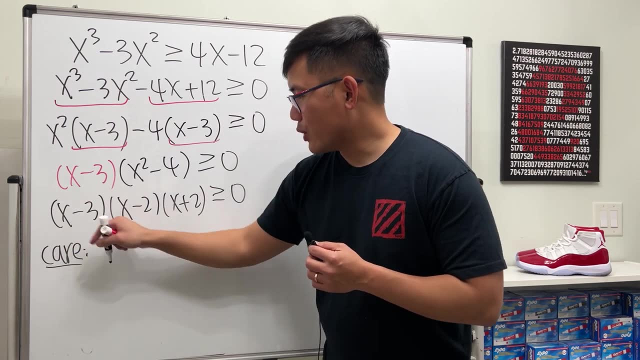 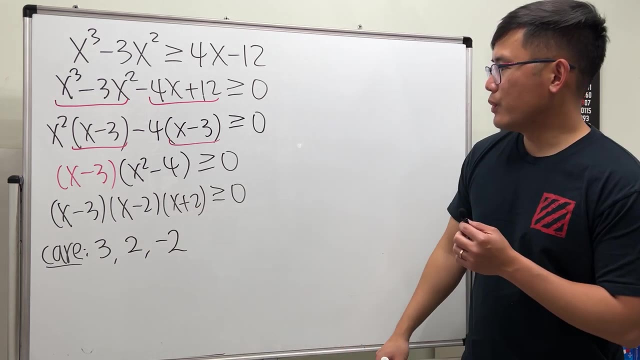 And this is greater than or equal to zero. Okay, so, what numbers do we care? Well, for this one, right here, we care about 3.. For this, right here, we care about 2.. For this, right here, we care about negative 2.. And here we go. Let's actually do the number line test. 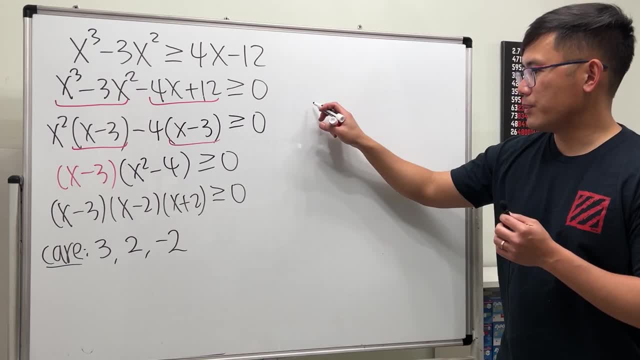 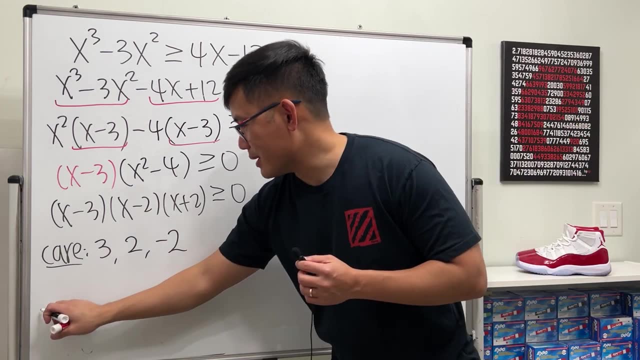 right, here We are looking for this thing. Yeah, so I'll okay, I'll write it down here. No, let's just do here, It doesn't matter. All right, let's put negative 2 here. Let's put 2.